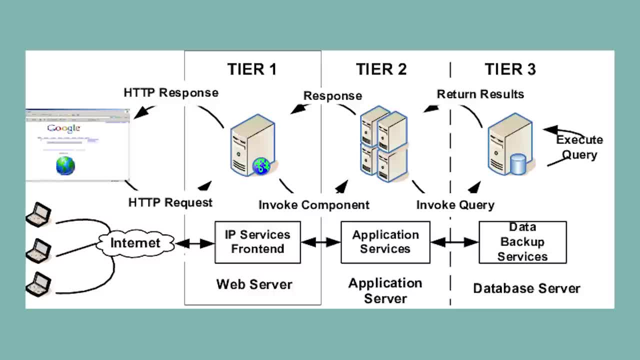 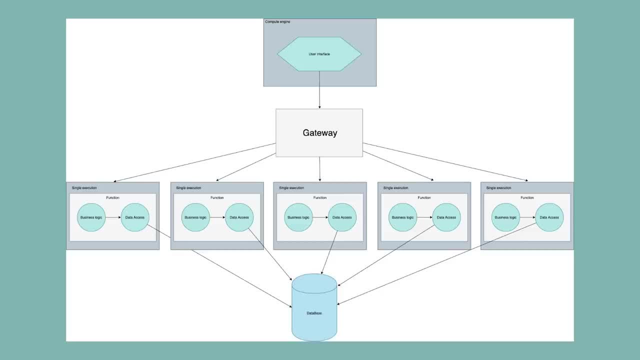 there is to consider in terms of architecture. I mean, how many tiers is your application? Where does each component live? All on the same server Or each have their own server? Are you going with a serverless architecture? And if you're on web 2, you're probably doing client-server. But if 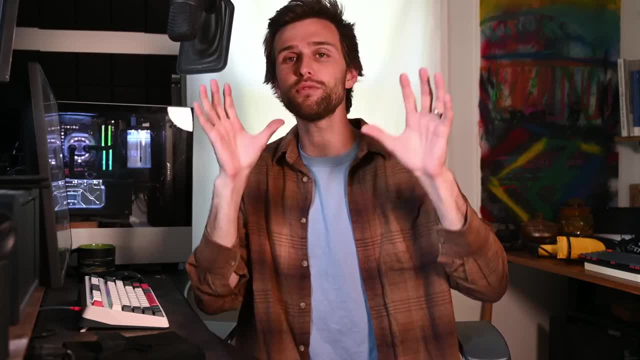 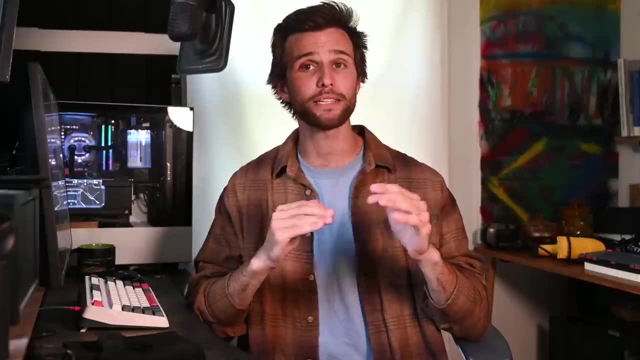 you're on web 3, then you're doing peer-to-peer. All of this matters in the context of what type of app that you want to build, So I've broken these down, put them into levels or buckets that are actually comparable and created explanations in a way for you to simply understand the. 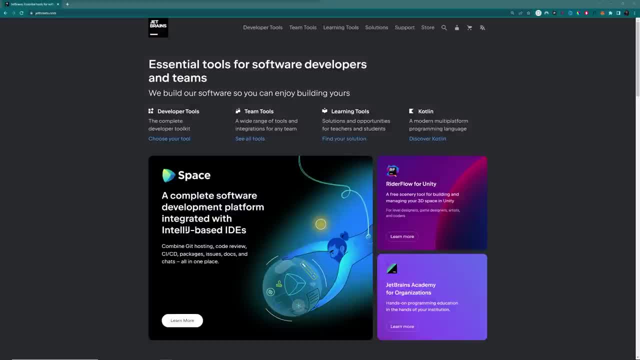 differences between the two. So I've broken these down, put them into levels or buckets that are actually comparable and created explanations in a way for you to simply understand the differences in the types of web app architecture. But first, I'm stoked to announce that JetBrains Space is the 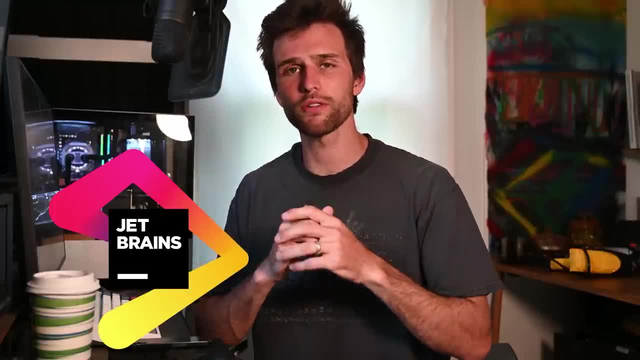 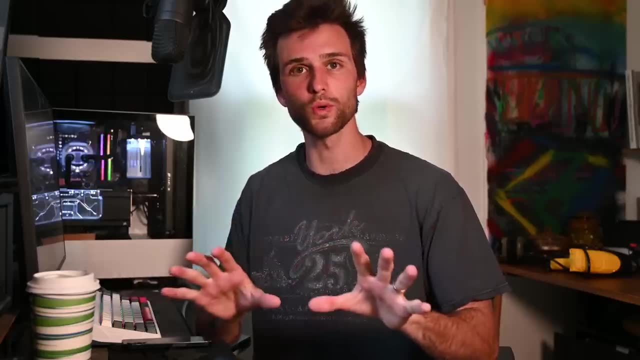 sponsor of today's video, And I may take a wild guess that you've already heard of JetBrains. They've created IntelliJ, IDEA, PyCharm, Rider, TeamCity and Kotlin, among many other tools for developers and software teams alike. But today I want to talk to you about a specific product. 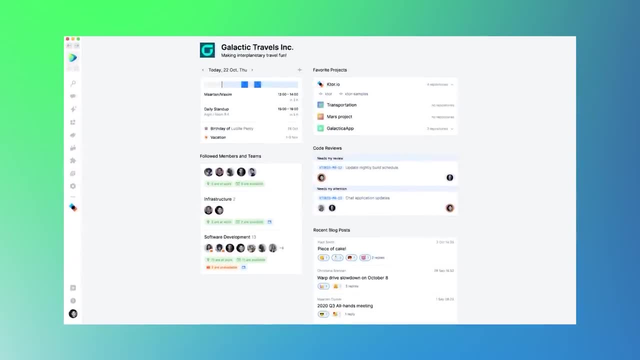 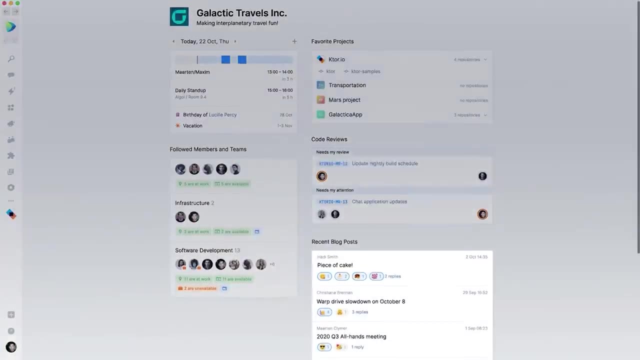 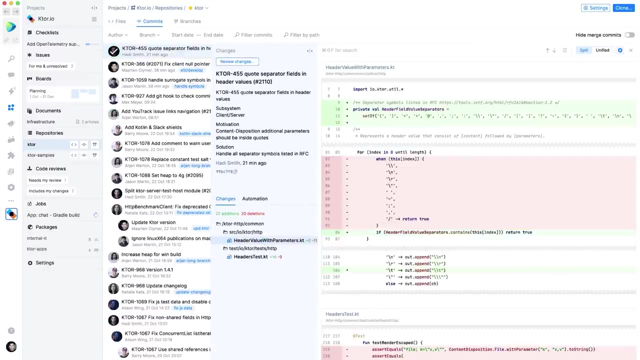 created by JetBrains. JetBrains Space Space is really a one-stop shop for all development tools. It's a unified platform that covers the entire software development pipeline- Everything you need in a single toolset: Source code control, hosting using Git code, reviews with merge requests and quality gates, automation, jobs for building and deploying. 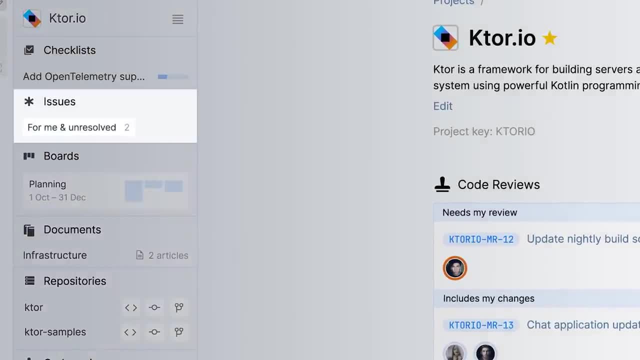 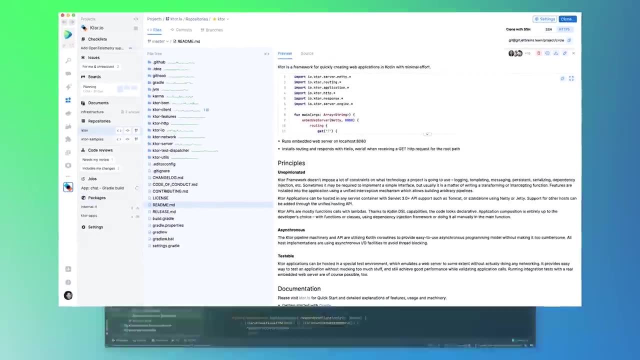 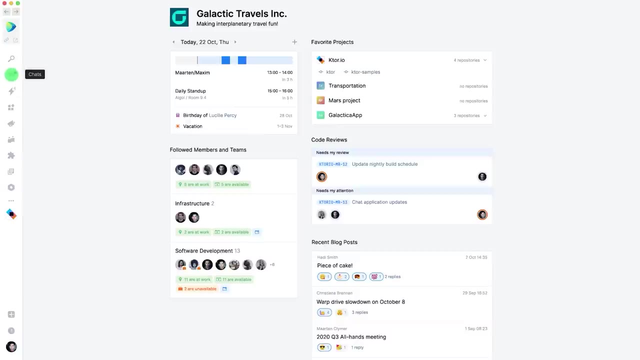 applications, project management tools, checklist for planning, an issue tracker and visual boards, packaging container, registries for publishing artifacts, the first class integration with JetBrains, IntelliJ based IDEs and cloud development environment for remote development with JetBrains IDEs. But it's not only about the development aspect, it's also about the 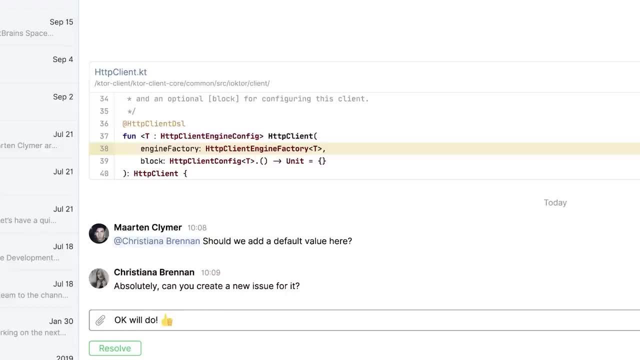 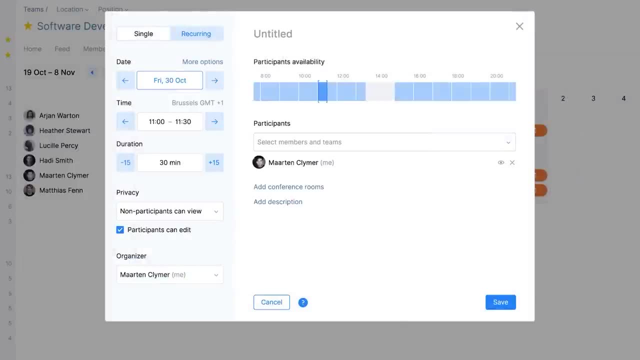 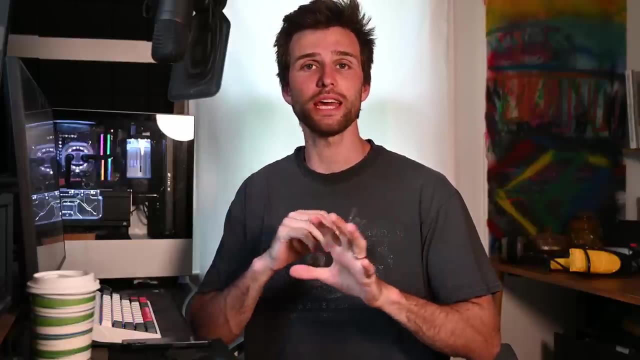 organizational and communication tools. You have a team directory for managing the company's organizational structure: management of vacations, absences and locations, chats, collaborative documents, blogs, meeting management, personal calendars and to-do lists for task management. So if you work in a team, especially if you use any JetBrains products, IDEs- I would heavily 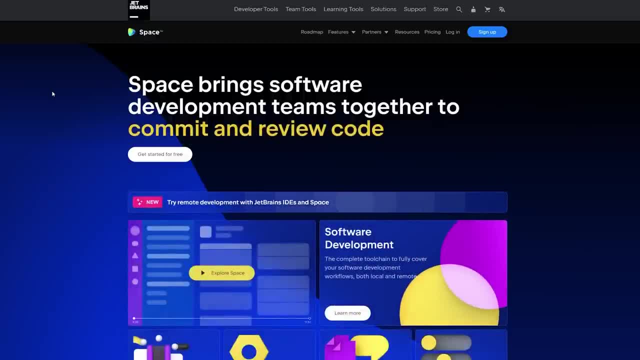 recommend checking out Space, because it puts everything you need for communicating and collaborating with your team in one place. You can try it out for free using my link in the description, but you can also upgrade to your favorite platform. So if you're looking for a 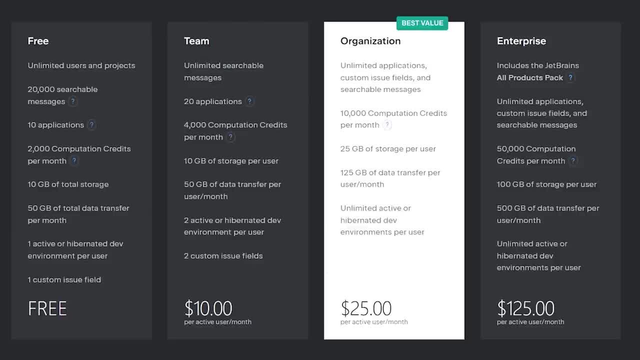 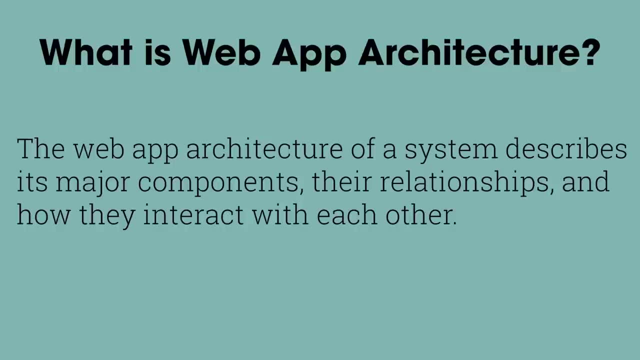 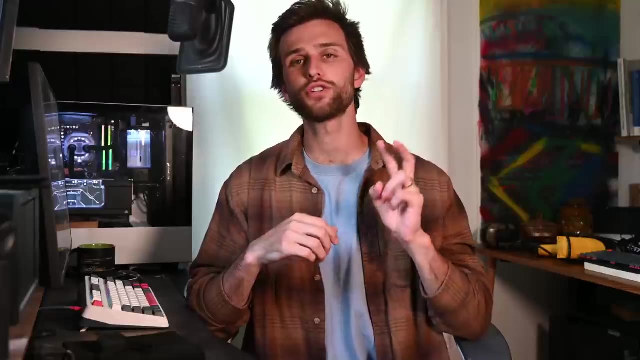 space team using my code, which is also in the description just below the link. So what is web app architecture? To put it simply, the web app architecture of a system describes its major components, their relationships and how they interact with each other. It essentially serves as a blueprint, the layout of it all, And there are two main ways in. 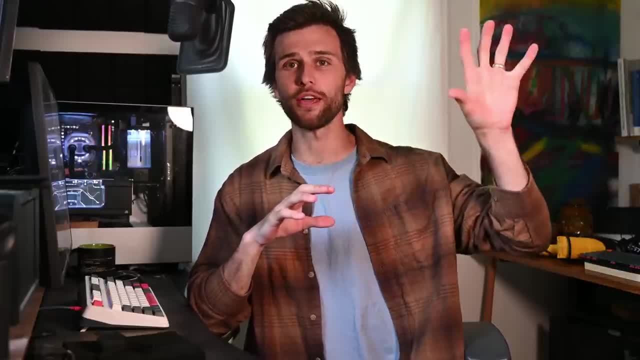 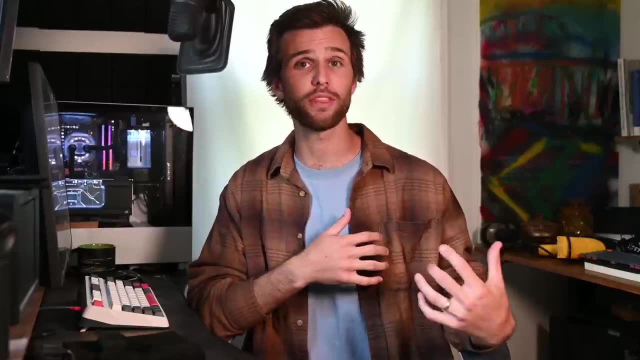 which it's laid out at least in the overarching more broad idea of architecture, with the main one being client-server architecture. It would be irresponsible for me not to start with this, as it is a fundamental building block of the web. So let's take the web app We typically have. 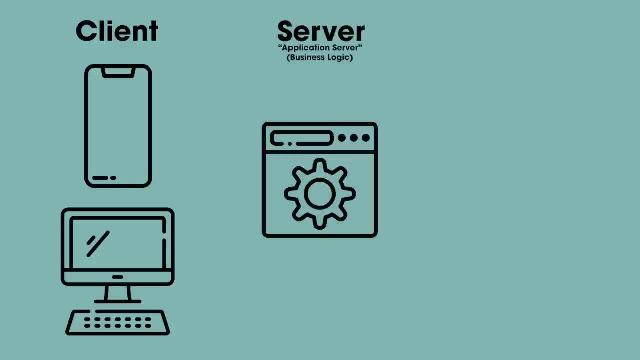 the client-side or front-end, the server-side or back-end, the database and everything in between. And not all web applications are set up just like this, where you have the client-side, the server-side, which is the business logic in this case, and then the database. 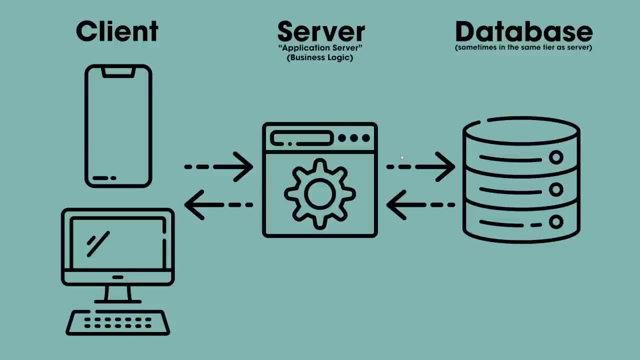 all living on their own physical machines. This is where different tiers in software architecture comes into play. A one-tier application will have all of this on a single machine. A two-tier application will have all of this on a single machine. A three-tier application. 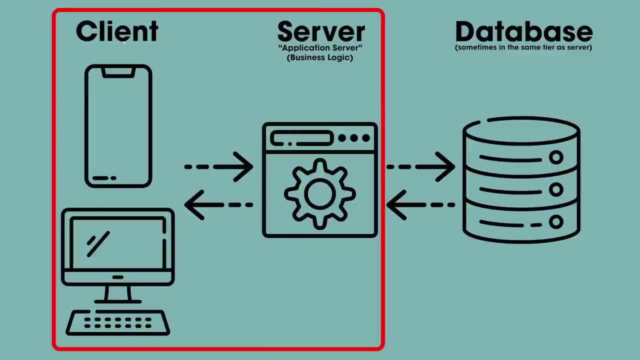 will have all of this on a single machine. A four-tier application will have all of this on a single machine. A two-tier application can be split one of two ways, with all of the code, so the client- side and then the server-side, business logic living on one machine and the database living 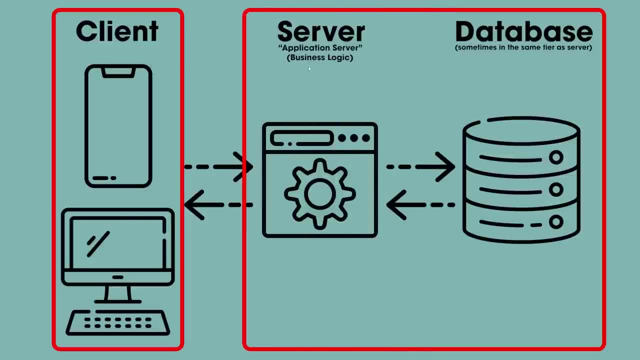 on a second machine, or the client-side living on one machine and then the server-side- business logic and database- living on the second machine. That's two-tier. What you're looking at now is three-tier, with each individual section being in its own machine. And finally, 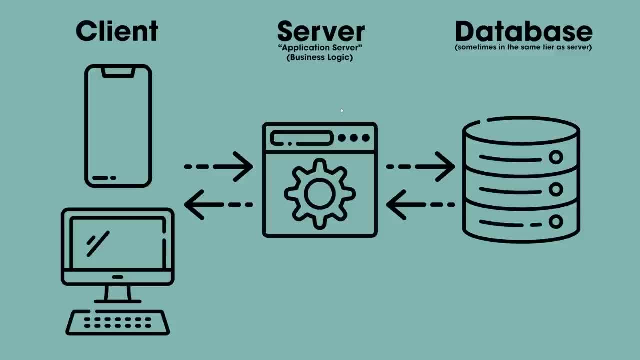 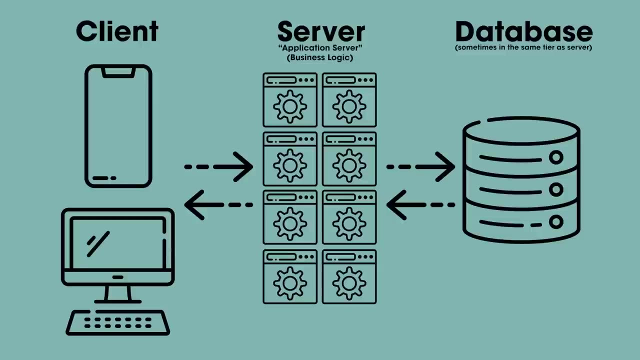 you have n-tier, which is anything more than a three-tier application. This typically takes into consideration the single responsibility principle, where each individual component lives on its own machine. So if you have five or ten different components, in terms of business logic you're going to have five or ten different machines just to cover this. 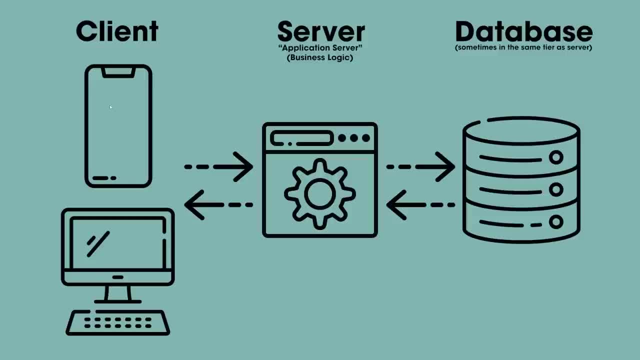 And for this example, we're sticking with a three-tier application. So on the client-side, as you interact with the web application, it'll send an HTTP request to the server, the business logic, which will then query the database if needed, which will respond with that data, which. 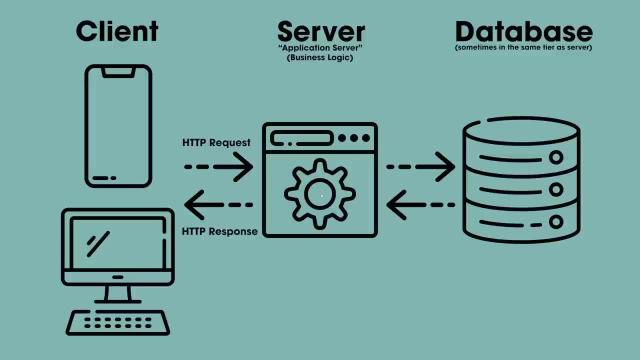 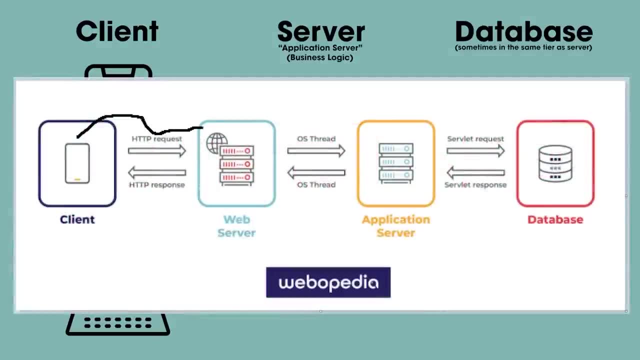 then we will transform that data as needed to send an HTTP response back to the client. And I will say, for all of the well-actualies that'll be in the comments section, saying: well, actually you send the HTTP request to a web server, which then sends an OS thread to the application server. 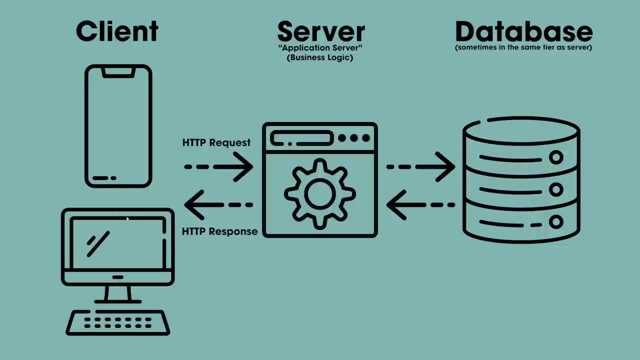 then does all of that and back through. Actually, you're speculating there. However, by strict definition, web server is a subset of an application server, So all of that occurs in our server-tier right here. Now let's take YouTube as a real-world example. 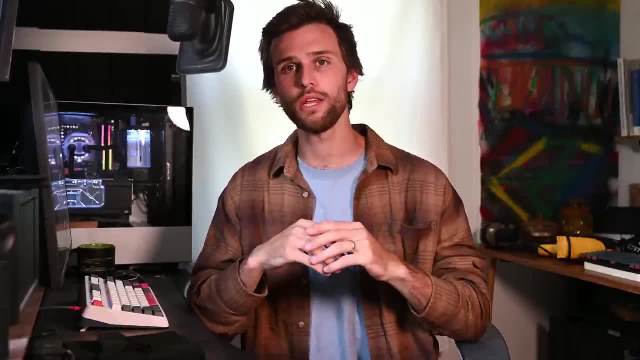 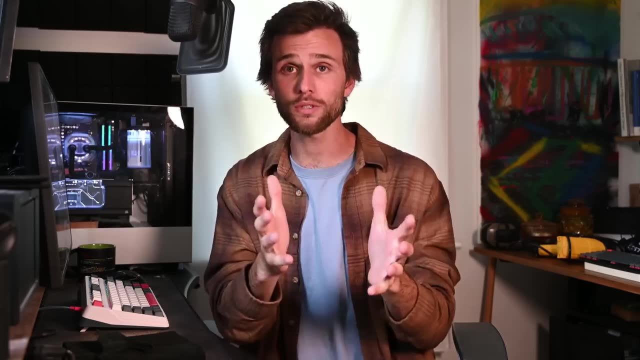 When you were on youtubecom and you saw this video pop up and you clicked on this video, you sent an HTTP request from the client-side, which is what you see- server-side, which is what you don't see, unless something has gone terribly wrong. 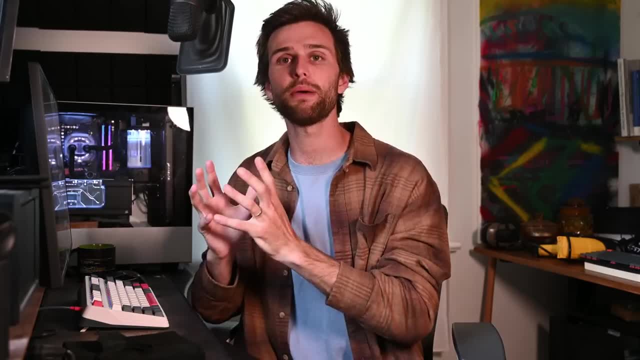 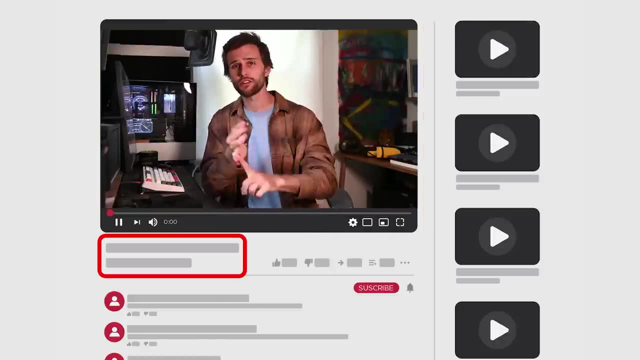 in order to access the business logic, the database and everything that you need in order to populate the webpage that you're on right now, which contains the video, the description, all of the metadata, the comment section, the recommendation system on your 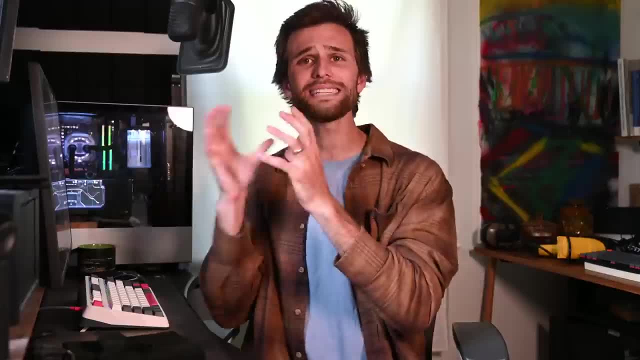 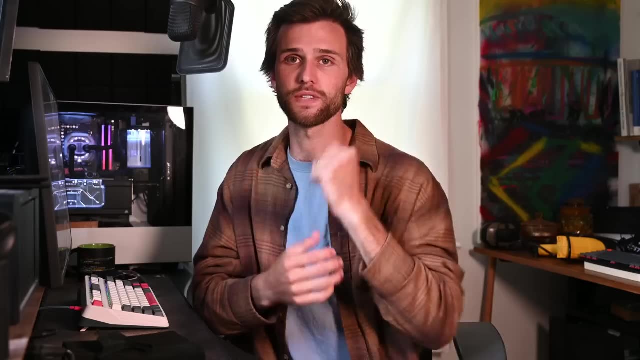 well, that side, I think everything that you see right now. It accesses all of that information and then responds back to the client-side with that information and serves it to you Basically every website you use- YouTube, Facebook, Twitter, your banking app. 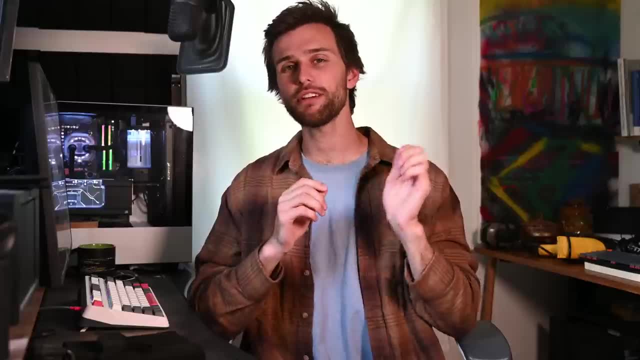 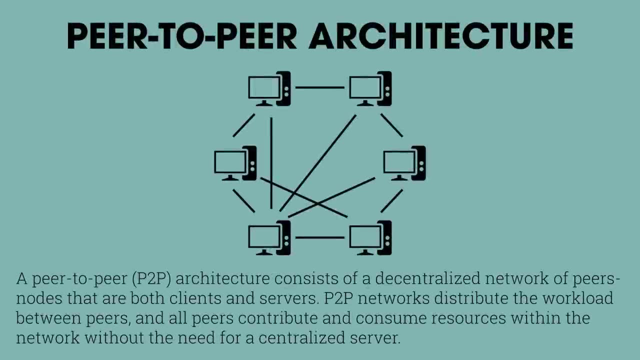 is all client-server architecture. However, there is something that opposes client-server architecture and that is known as peer-to-peer architecture. There are a small percentage of businesses that use this, and I'll give you some examples, but something that you can really wrap. 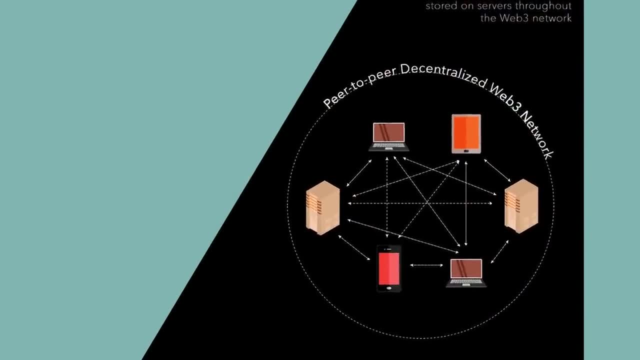 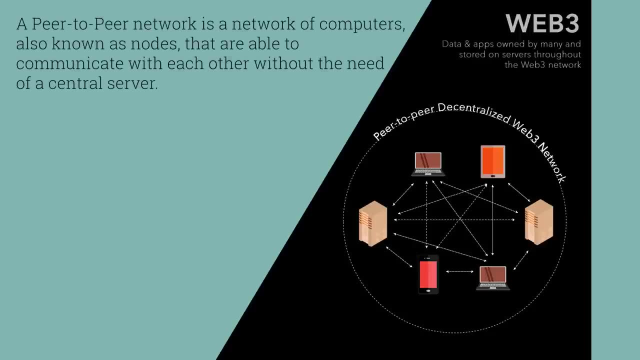 your head around is Web3, the blockchain. Peer-to-peer architecture is the base of blockchain architecture. It is a network of computers, also known as nodes, that are able to communicate with each other without the need of a central server like that of client-server architecture. So it 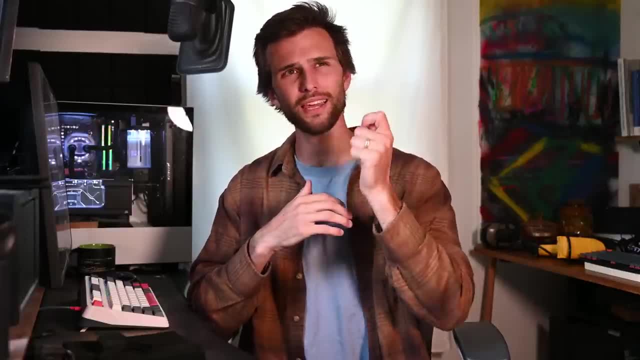 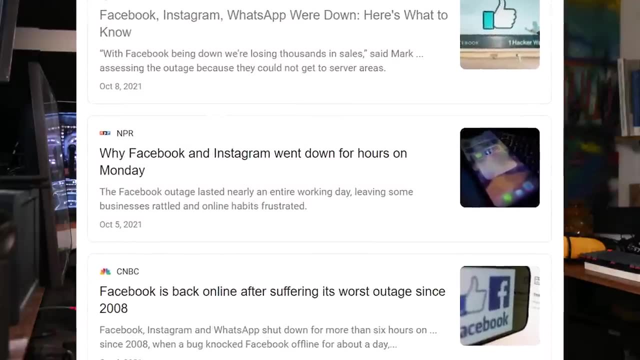 rules out the possibility of single-point failure, which I think. I don't know if it was earlier this year or in 2021,- when Facebook and everything that Facebook owned- WhatsApp, Instagram- went down for a day because their servers failed. That is one of the negatives of client-server. 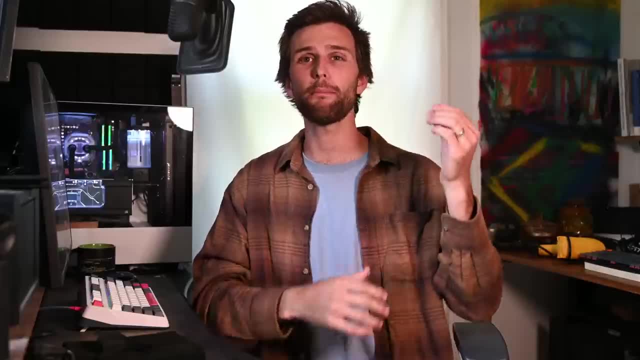 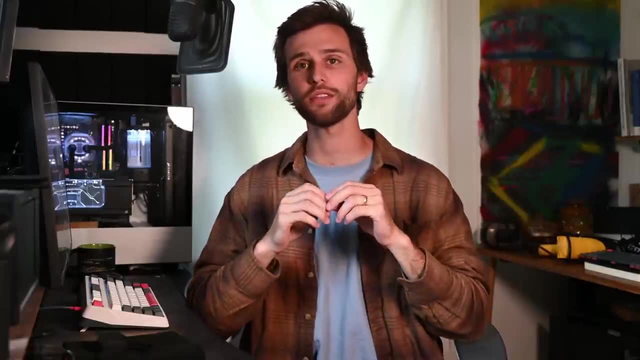 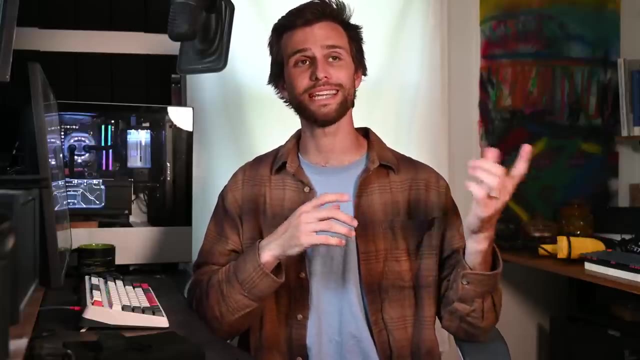 and one of the avoidances or solutions that peer-to-peer provides. Peer-to-peer technology, however, is not only used in Web3 and blockchain technology. It actually exists currently with some online gaming platforms. For example, Blizzard uses peer-to-peer to download games between users. They use this for Diablo 3,, Starcraft 2, and WoW, But for the 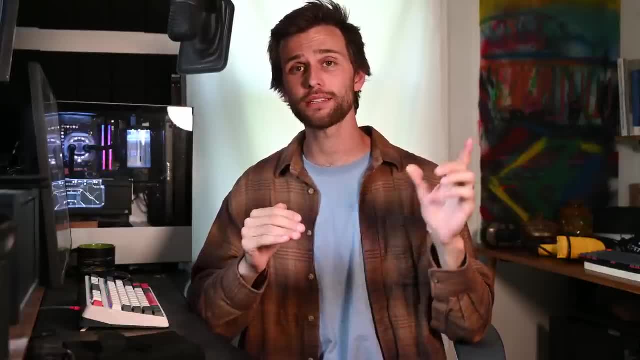 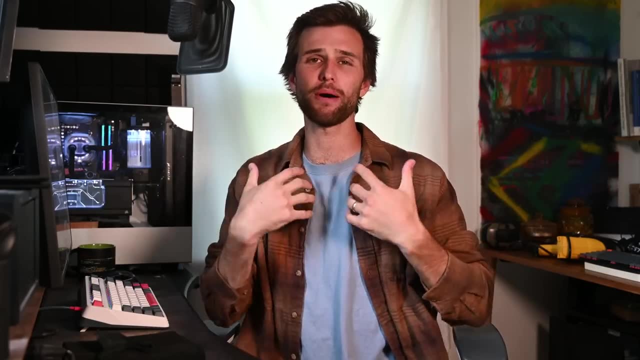 vast majority of what the internet is today, it is client-server architecture. So now we have the next level of architecture. Again, these are levels created by myself. I just wanted to be able to get to the bottom of this and give you architecture that is actually comparable to each other. 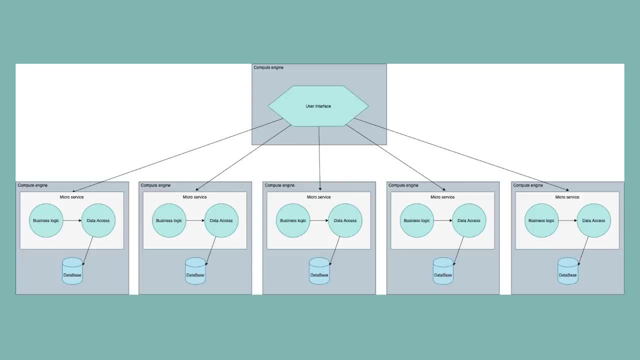 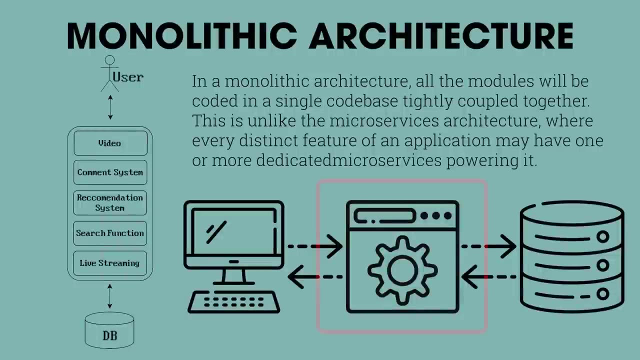 and not just a bunch thrown in your face. So this is where monolithic microservices and serverless come into play. In a monolithic architecture, all the modules will be coded in a single codebase, tightly coupled together. This is unlike the microservices architecture. 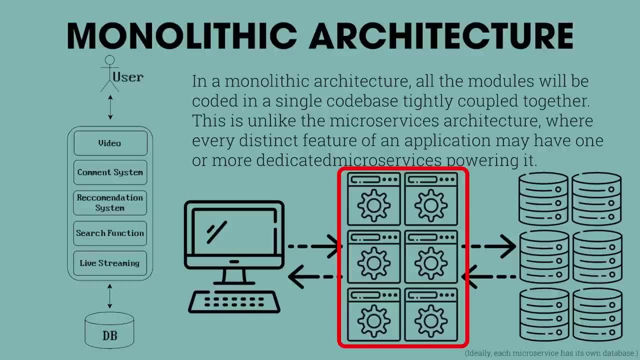 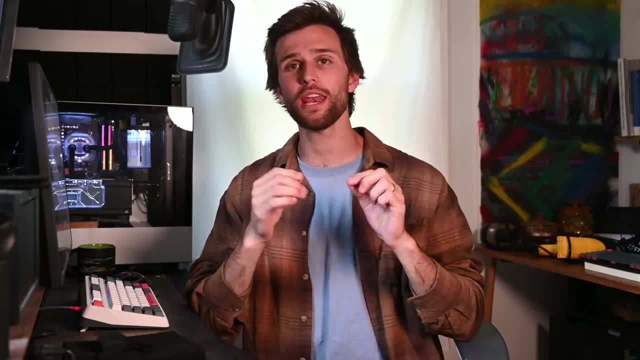 where every distinct feature of an application may have one or more dedicated microservices powering it. This is how basically everything used to be built, Because it's I mean, it's simple, it's fast, you can easily deploy it. However, there are a lot more negatives than there are. 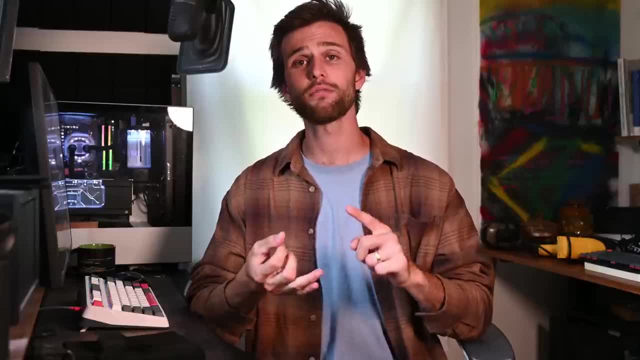 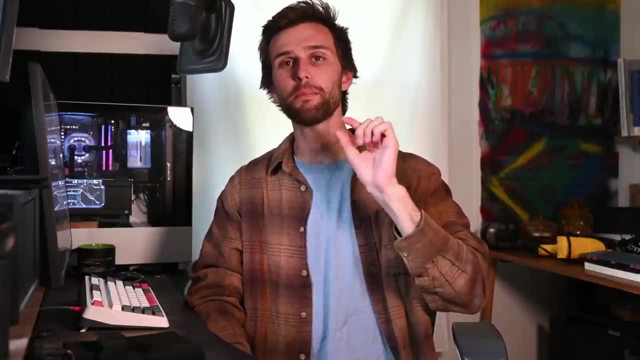 positives, because it's not scalable, It's not reliable. There are single points of failure To put in perspective. every single time you add a single line of code, you would have to redeploy the entire application. And not only do you have to redeploy it, but if something breaks, 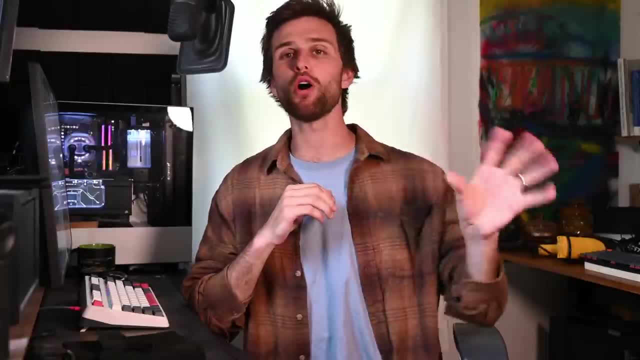 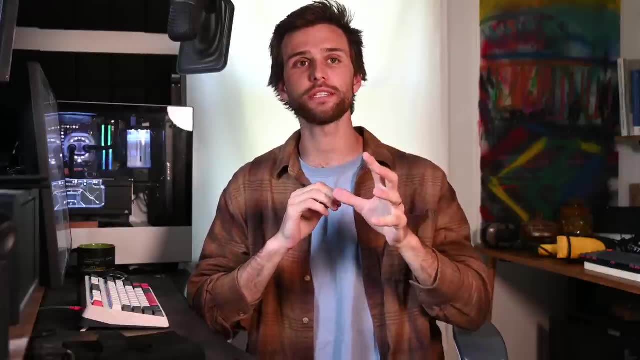 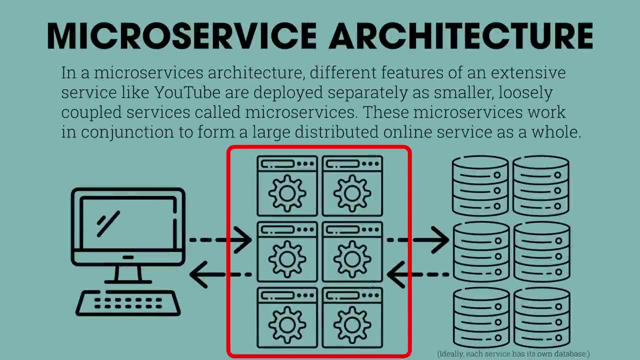 it breaks the entire application. However, the answer to all of those problems is solved with microservice architecture. This is where you have a collection of services that each serve a unique responsibility. Every single service is deployed and lives separately from one another. And to complete the business, 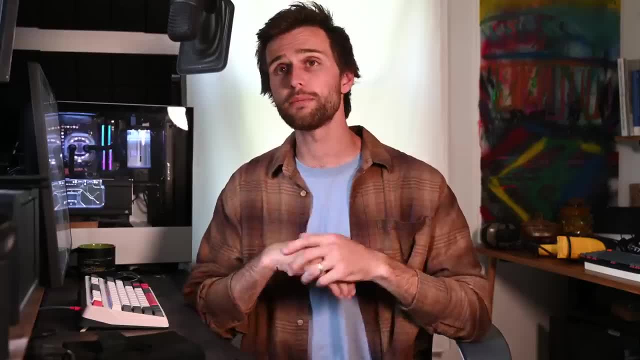 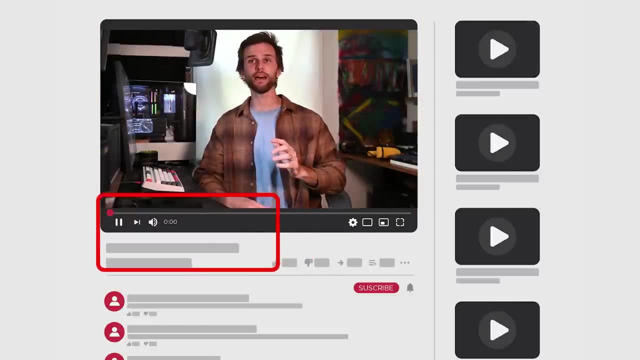 logic, they can connect to each other as needed, Or, to put it simply, it's modular. So where you have all of these different aspects of YouTube that you can see on your page right now, you have a software development team that works on one service: the recommendation system, And 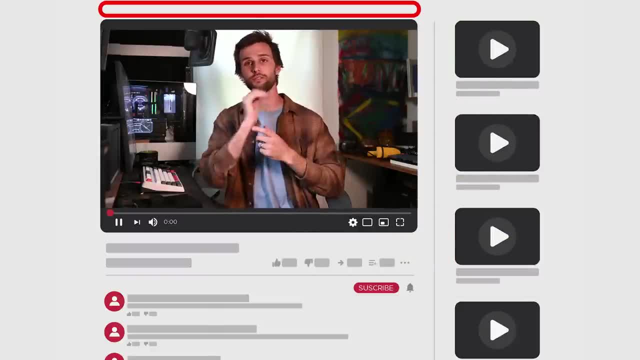 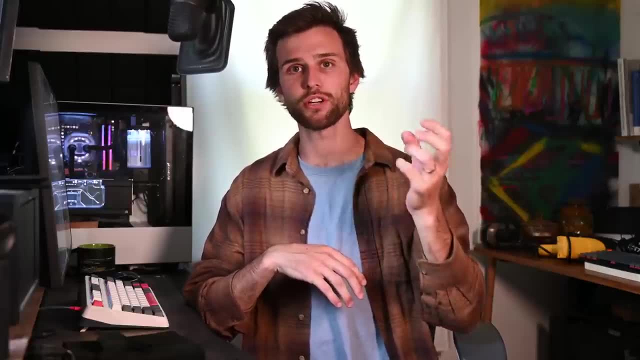 then you have another team that works on another service, the search function. Then you have another team that works on the comment system, so on and so forth. If they change one line of code, they're only redeploying their service, not the entire. 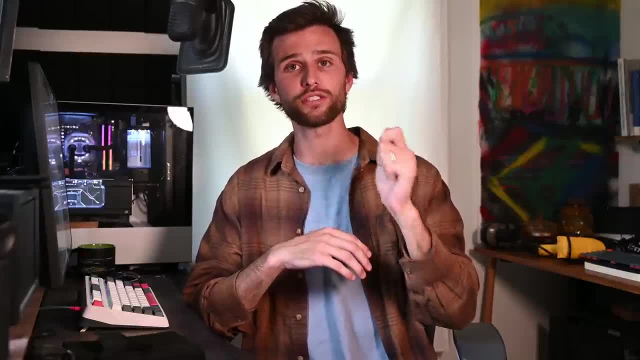 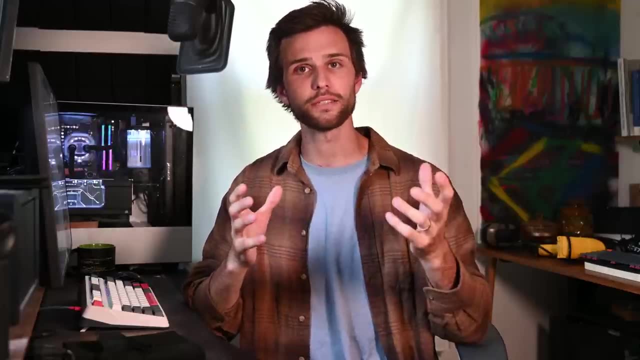 app And if they break something, they are breaking only their service, not the entire app. And then, of course, with it being modular, you can see just how scalable it is, because each service can be scaled independently, based on traffic And where there is monolithic architecture. 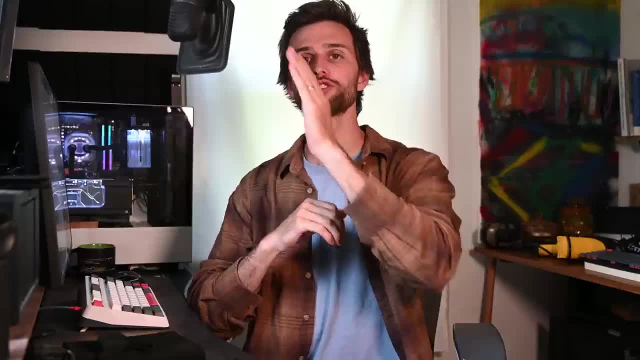 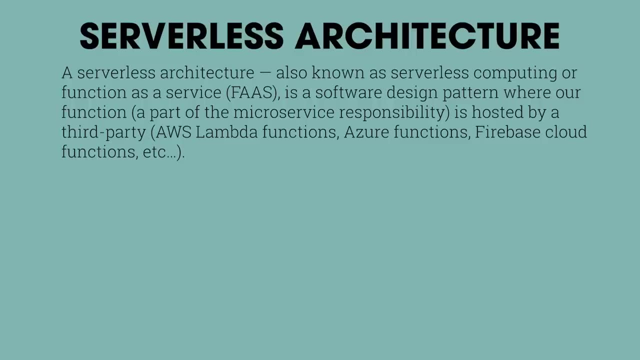 and microservice architecture. there is also something called serverless architecture, also known as serviceless, serverless computing or function as a service. It's a software design pattern where our function, which is a part of the microservices responsibility, is hosted by a third party. This is your AWS Lambda functions, your Azure functions.